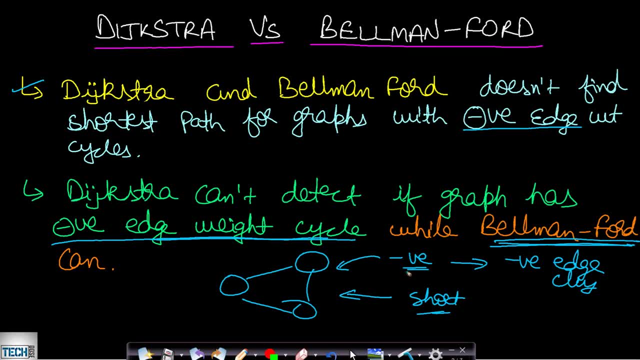 we will be using bellman ford algorithm. otherwise, if we use dixtra algorithm, then even if the graph is having negative edge weight cycle, still it will give you the shortest path answer and that answer may be wrong. okay, so whenever you are looking at dixtra and bellman ford algorithm, then you should. 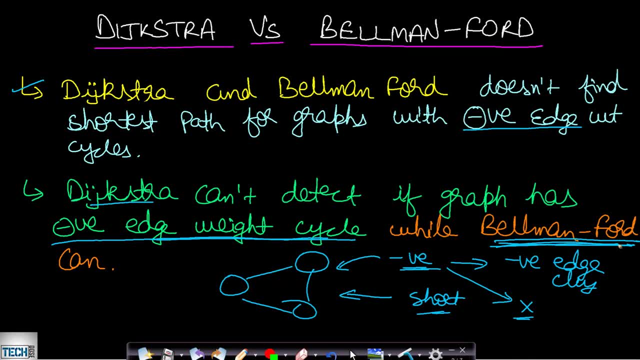 make sure that you are using bellman ford algorithm because in this case, if your graph can have negative edge weight cycle, you will be using this bellman ford algorithm. this will be having some higher complexity as compared to dixtra, which i will be showing you at the end of the video. 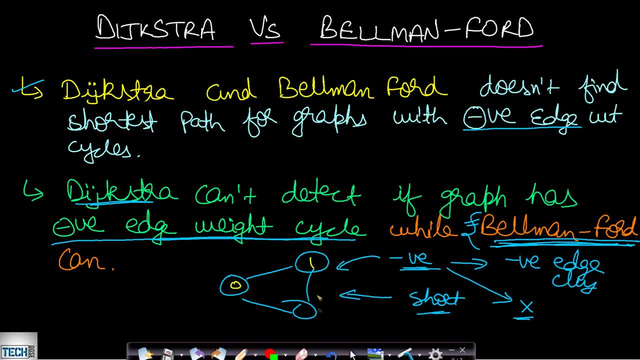 now, what is an negative edge weight cycle? let's say your graph is having three nodes- zero, one and two- and the edge weights are given as 2, 3 and minus 6. then in this case, if you start from zero and again come back to 0, then what will be the cost? the cost will be equal to two plus three plus. 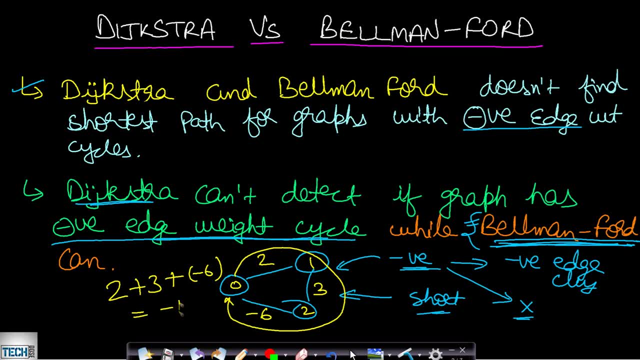 plus minus 6, and this will come out to be minus 1. you can see that the cost is negative. this indicates that you are not really spending anything, but you are getting a benefit of one unit. so this is a negative edgeward cycle. if, instead of this minus 6, let's say we had minus. 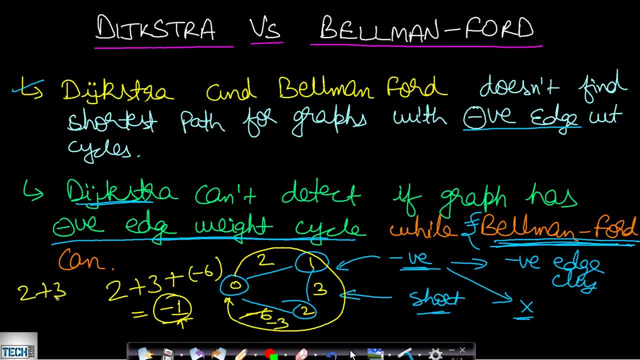 3, then the cost would have been 2 plus 3 plus minus 3, so the total cost would have come out to be 2. so this is not a negative edgeward cycle, because the total cost is positive. okay, so i hope you understood the difference between what a negative edgeward cycle is and what a positive. 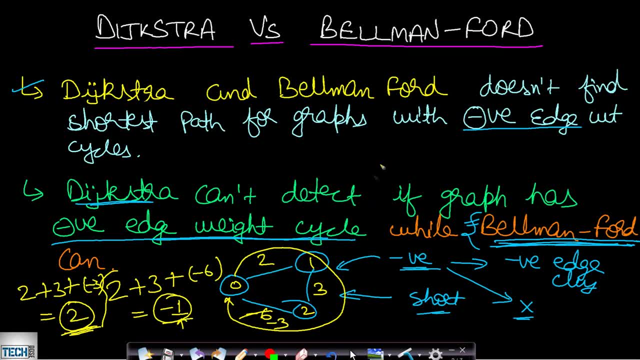 edgeward cycle is. so in this case you can see that just by having a negative edge weight, you cannot say that you will be having a negative edgeward cycle. okay, so for this graph, having weight 2, 3 and minus 3, dijkstra algorithm will also give you the correct answer. 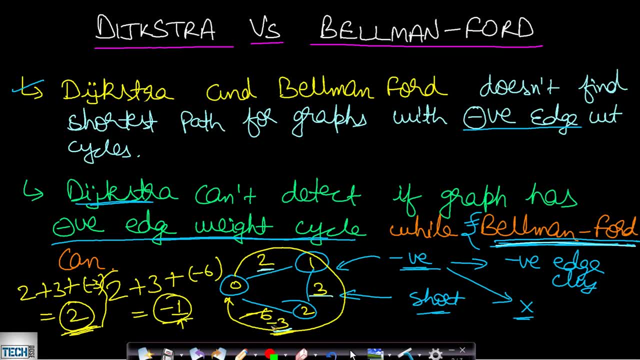 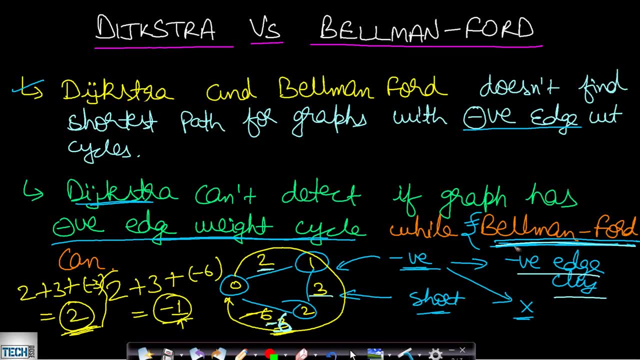 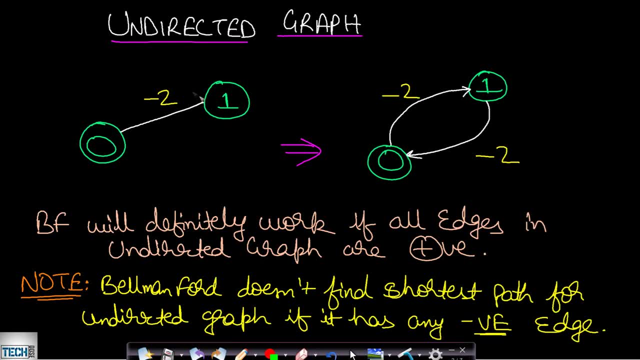 have given you a wrong answer, so that is why we will be using the bellman ford in such cases. now i hope you understood the comparison of dykstra and bellman ford. now there are two types of graph: undirected graph and a directed graph. so there is a special case for undirected graph. 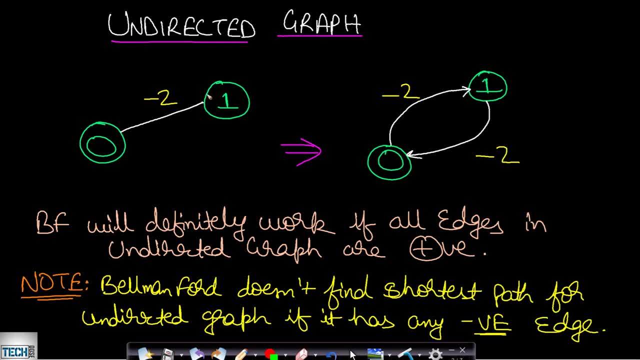 in undirected graphs. if you have a negative edge weight, then definitely there will be a negative edge weight cycle in the graph. so let us assume that our graph is having just two nodes, this 0 and 1. then in this case, if you have an edge from 0 to 1, an undirected edge, then this is as good. 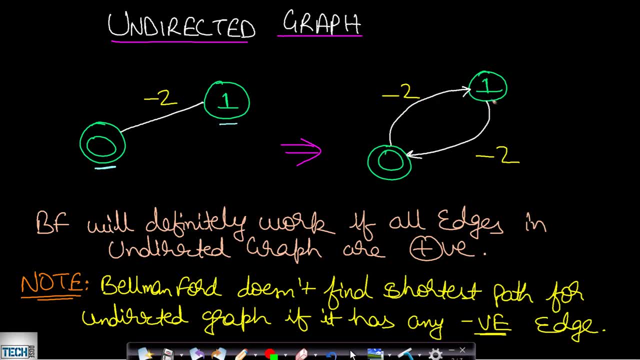 as saying you have a directed edge from 0 to 1 as well as a directed edge from 1 to 0. if your edge was minus 2 here, then from 0 to 1 you will be having weight of minus 2. from 1 to 0 you will. 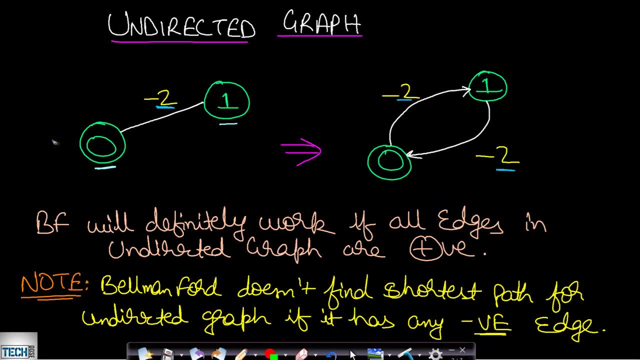 0, you will be having a weight of minus 2. okay, now, if your source is this 0 and your destination is this 1, then the cost from this source, the source will have cost 0. from source to this destination, the cost will be minus 2. now, if you want to calculate the cost from 1 to 0, then it will come. 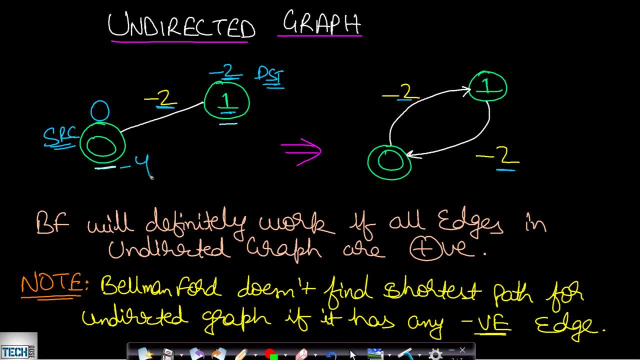 out to be minus 2 plus minus 2, which will be minus 4 again. if you find the minimum cost from 0 to 1, then this will come out to be minus 4 plus minus 2, which will be minus 6. so since minus 6 is smaller, 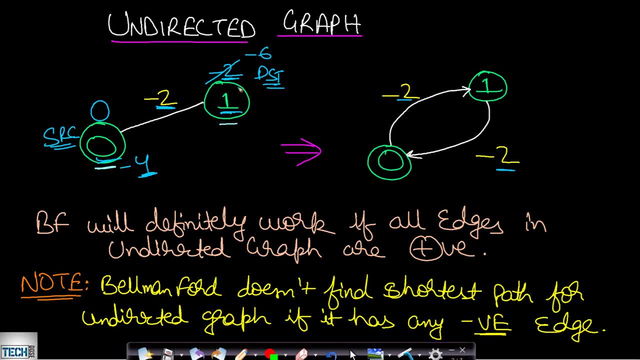 it will be replaced and this will turn into an infinite loop. okay, so this is why, if your undirected graph is having a negative edge, then that will surely mean that you are having a negative edge weight cycle. okay, so this is very simple: that if you have an undirected graph and 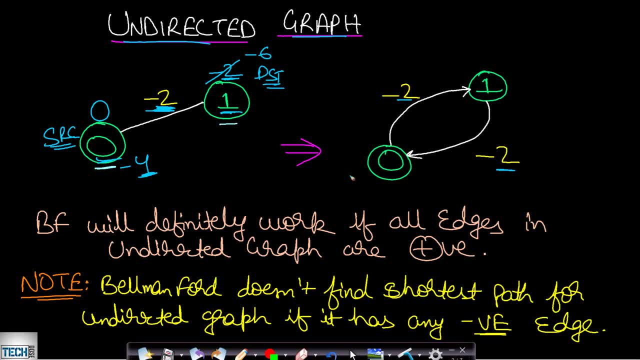 you have a negative edge weight, then that will have a negative edge weight cycle and this will indicate that your dixtra, as well as your bellman ford, will fail. so in such type of undirected graphs you can first check if your entire graph is having any negative edge. if it is true, then 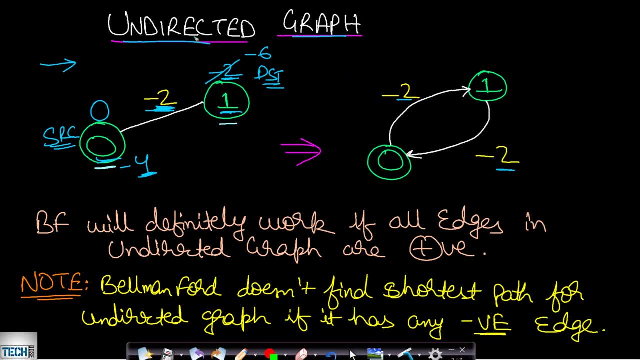 you cannot apply the shortest path algorithm. otherwise, if all the edges are positive, then you can definitely apply shortest path algorithm. okay, so bellman ford doesn't find the shortest path for undirected graph if it has any negative edge. bellman ford will definitely work if all the 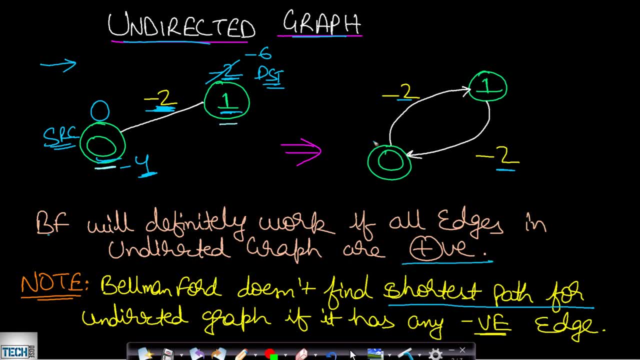 edges in undirected graph are positive. so if you have any negative edge weight cycle then you can apply shortest path program for undirected graph, if this isются to be the case are positive. so i hope you understood it. now, for the directed graphs, the complexity will be different, so i will 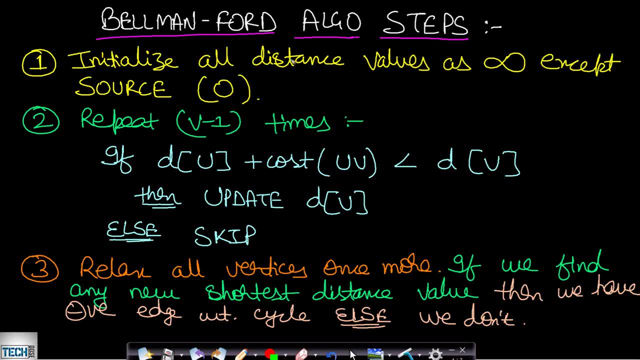 give you an example for directed graph. but before looking at the example, let us first look at the algorithm steps. so this is a three step process. in the first step we will initialize all the distance values with infinity, except the source, as zero, because the cost from source to source 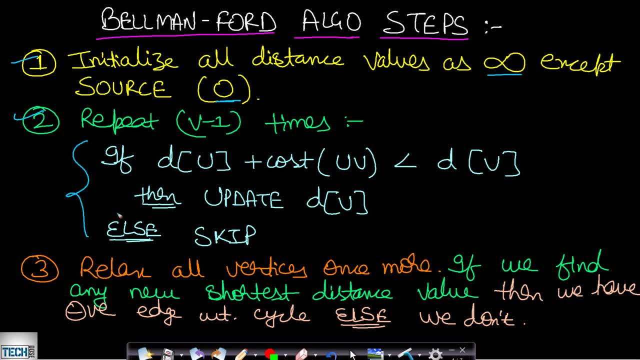 will be zero. now we will be repeating the steps of relaxation v minus one times. so we will be basically starting from this source node and we will be relaxing all the adjacent vertices. and why are we repeating these steps v minus one times? let's say you have three nodes. 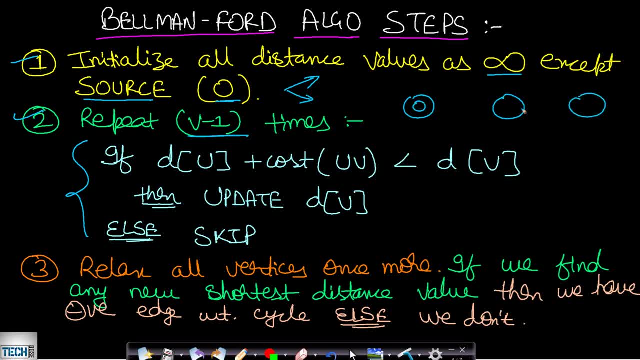 then what will be the minimum number of edges in order to reach to two? from one it will be equals to two, okay, which is nothing but v minus one. now, this is the minimum number of edges you require in order to cover all the vertices. this i have already explained in mst algorithms link will: 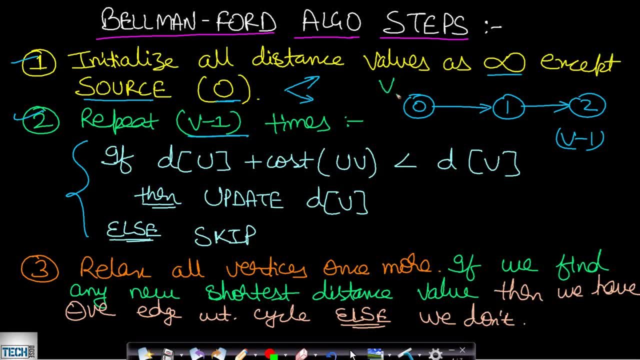 be present in the description below. so, similarly, if you have v number of vertices, then you will require v minus one number of edges in order to cover all the vertices. okay, so that is the reason we are repeating it: v minus one times. now, what will be done as a step of relaxation if we are 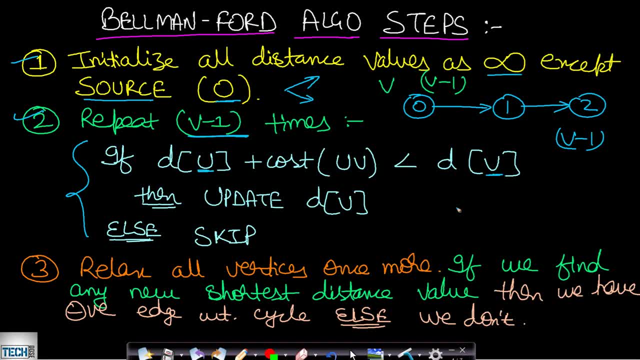 at a node u and we want to go to node v, that is, we have an edge from u to v, then this will be the minimum number of edges in order to reach to two. from one it will be equals to two. this node v will be updated with a new distance value if we have a certain cost at this node u. 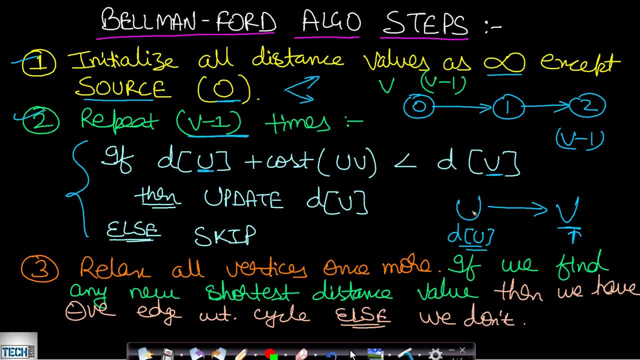 let's say it is d at u and we have a edge weight in order to reach to this v from u and that is equals to cost of uv. okay, so if the cost in order to reach to this u from some source is equals to du and the cost from u to v- that is, the edge weight- is equals to cost at uv. 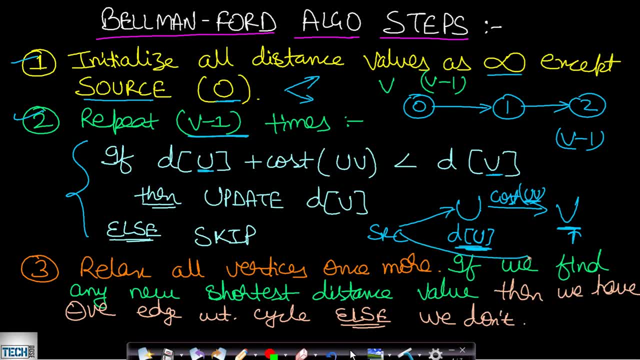 and the cost at v, that is, there might be some other path in order to reach to this v. so the cost to reach to this v was equals to dv. then if the new path is having a lower cost, then we will remove this path and we will add this new path, and so we will update the cost. 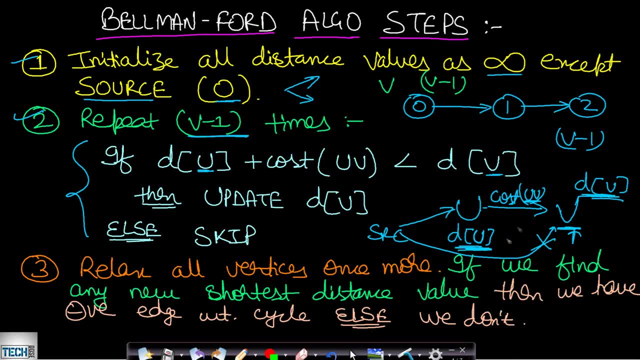 of d at v, which will be equals to d at u plus cost at uv. so this is the format which we will be using. this is the same format we have been using for the last time, so we will be using this format in all the previous algorithms as well. so i hope you will understand this easily now. if 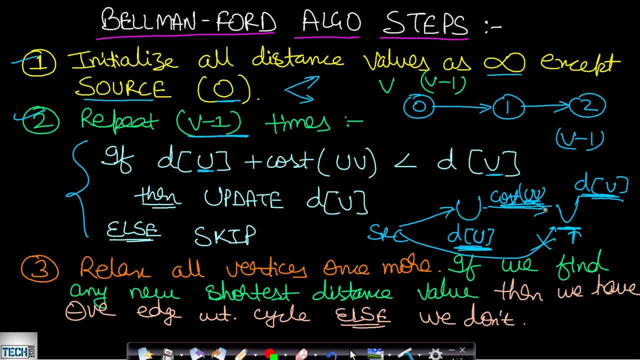 the cost of du plus cost of uv will be greater than dv, then we will not update it. okay, so we will skip it. this we will be repeating for v minus one times for all the v vertices. okay, so this will be done for all the v vertices. now the third step is, after doing all the relaxations, for all the 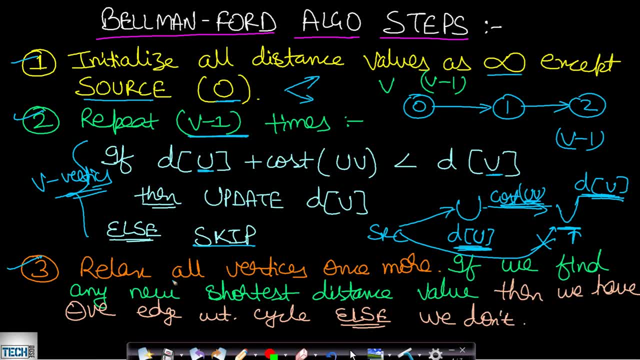 nodes v minus one times. we will check. if the node v is greater than dv, then we will not update it. so we will check if we have the shortest paths. so relax all the vertices once more and after relaxing once more, if we find any new shortest distance value, then we have a negative edge weight. 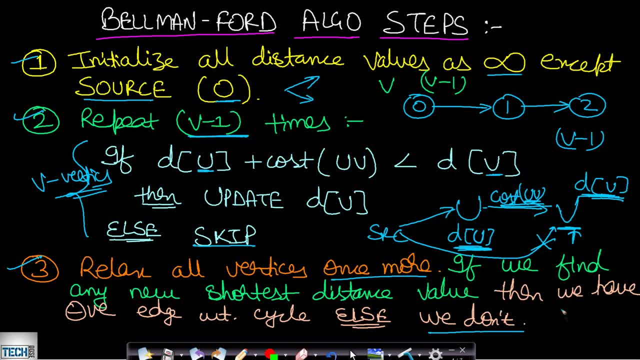 cycle, else we do not have any negative edge weight cycle and we can simply return the answer. so this i will be explaining at the end of the video, after explaining the algorithm. so let us now dry run the algorithm in order to get better understanding. so what was the first step? let us assume that our 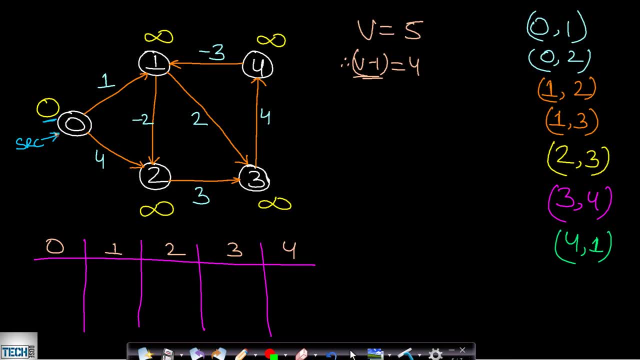 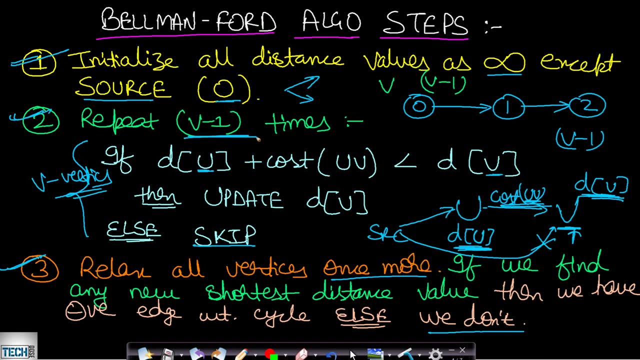 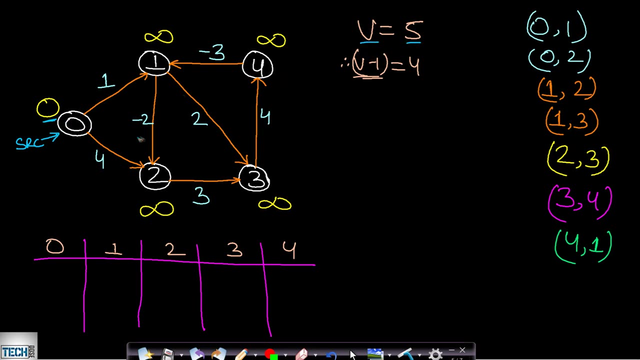 to zero. so our first step was to initialize source with distance zero and all the other vertices with infinity. so this was our step one. now for step two. we will be repeating for v minus one times. in this case we have v value equals to five, that is, nodes from zero to four. so v minus one value. 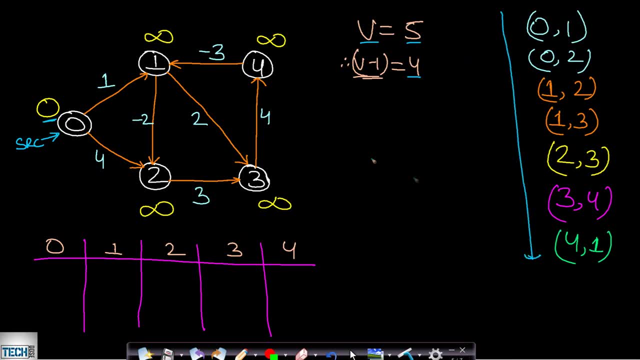 will be four. i have written all the vertices here, okay, and we will be relaxing all the vertices four times. so we will be starting from this source, node zero. it has cost zero. now, from this zero, if we want to reach to this one, then the cost will be cost at zero, which is zero plus the edge weight. 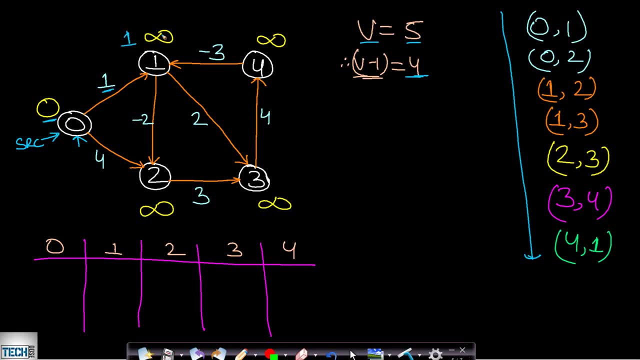 which is one, so this will be one. now, the initial cost was infinity, so since we have found a minimum cost, we will now replace it with one. so we will move to the next stage. it is zero to two, so, from zero to two, the cost will be zero plus four, which will be four, and the already present cost is 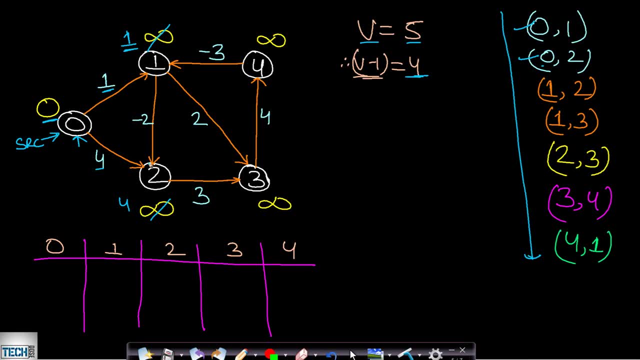 infinity, which is greater. therefore, we will be replacing the value for the cost, which is zero, 4. it will be replaced. now. this 0, 2 is relaxed. we will move to 1, 2 now from 1, 2 or this 2, the cost. 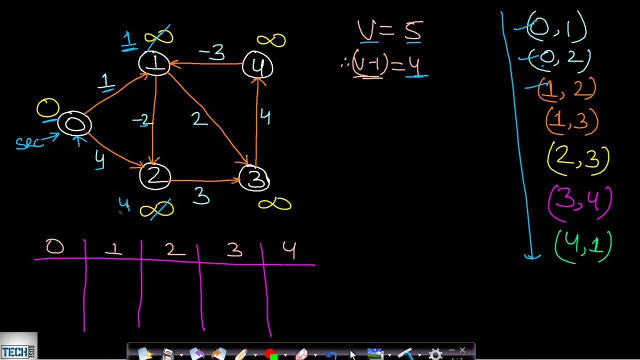 will be 1 minus 2, which will be minus 1, so the already present cost is 4. it will be replaced with minus 1. okay, so 1, 2 is now relaxed. we now see this. 1, 3, from 1 to 3, the cost will be 1 plus. 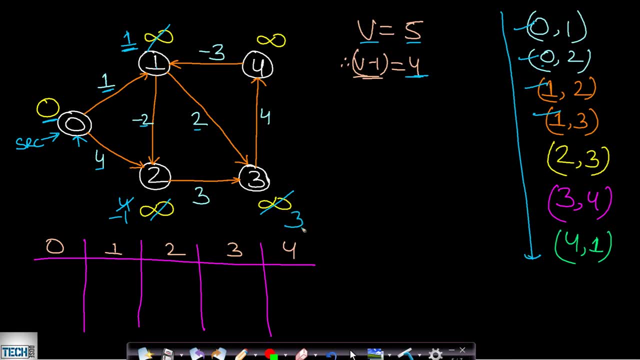 2, it will be 3. so 3 is lower than infinity, so it will be relaxed. now we move to 2- 3. so 2 to 3, the cost will be minus 1 plus 3, which will be 2. so 2 is lower than 3. so this will become 2. now we 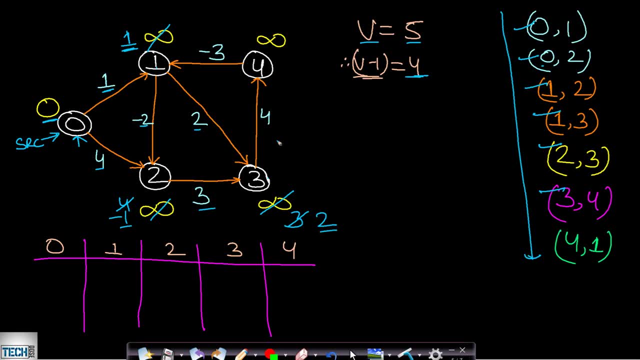 relax this: 3 to 4. from 3 to 4, the cost will be 2 plus 4, which will be equals to 6, and 6 is lower than infinity, so this will be replacing it now. from 4 to 1, the cost is minus 3, so this will be. 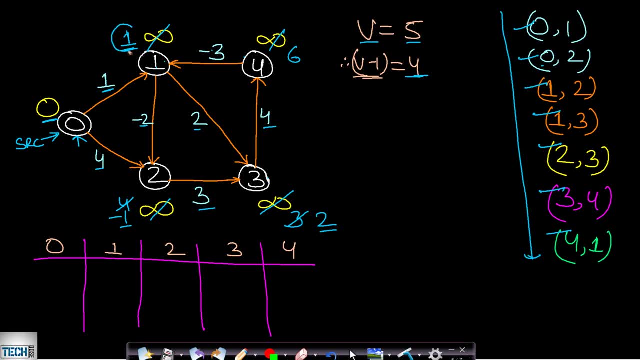 6 minus 3, which will be 3, but the already present cost is 1, so we will not replace it, okay? so all the edges have now been relaxed and we have relaxed for the first time. so let us now write all the cost after one time relaxation. so 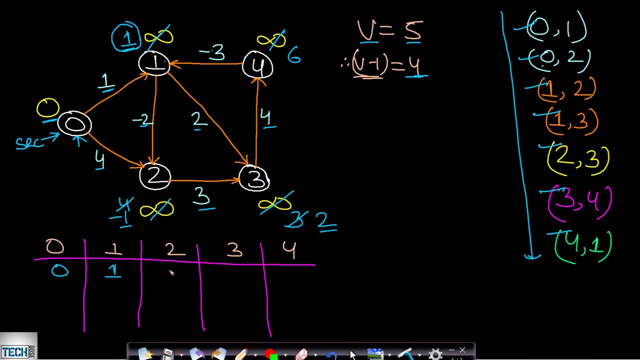 0 is having cost 0, 1 is having 1, 2 is having cost minus 1, 3 is having cost as 2 and 4 is having cost as 6. okay, so this is for the first time. relaxation now. what about the second time? we will have to. 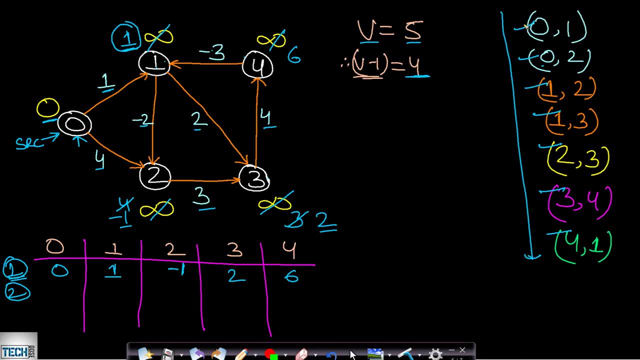 repeat for four times. so again, we will be starting for this 0- 1. so if we relax 0 to 1, the cost will be 0 plus 1, and already present cost is 1. so this will be the same now for 0 to 0 to the cost will. 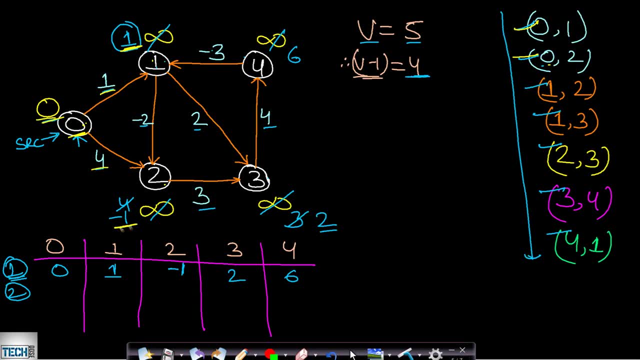 be 0 plus 4, which will be 4, but already present cost is minus 1. so it will not be replaced for 1- 2. from 1 to 2 the cost is minus 2. so if you see 1 minus 2 is minus 1, it is already minus 1. 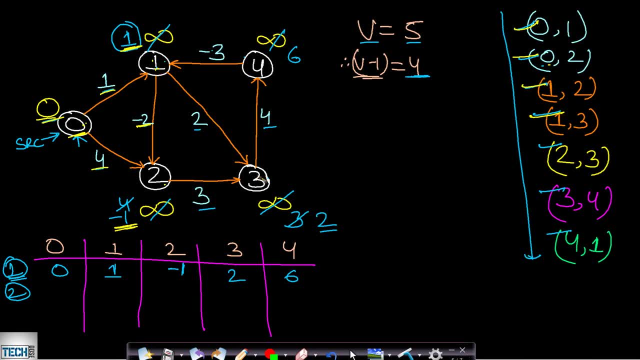 nothing will be done now for this. 1- 3. from 1 to 3, the cost is 2. it will be 1 plus 2, which will be 3. so already present cost is 2. so this is minimum. we don't need to do anything now for this. 2 to 3. 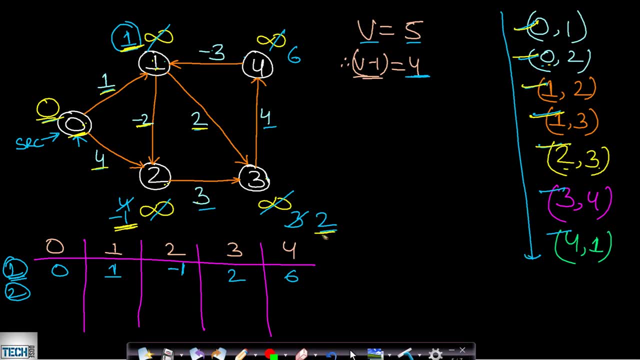 2 to 3, the cost is minus 1 plus 3, which will be equals to 2, and 2 is already present, so it's perfect. now for 3 to 4. 3 to 4, the cost will be 2 plus 4, which will be equals to 6. 6 is already. 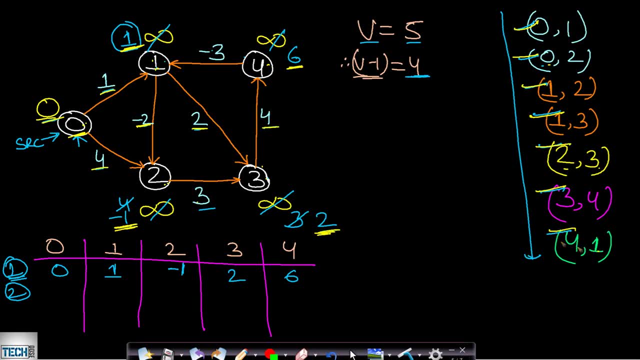 present, we don't need to do anything now. for this one, 4 to 1, the cost will be 6 minus 3, which will be 3, so already present cost is 1. okay, so nothing will be done. you can see that we have relaxed all the edges once more and the cost. 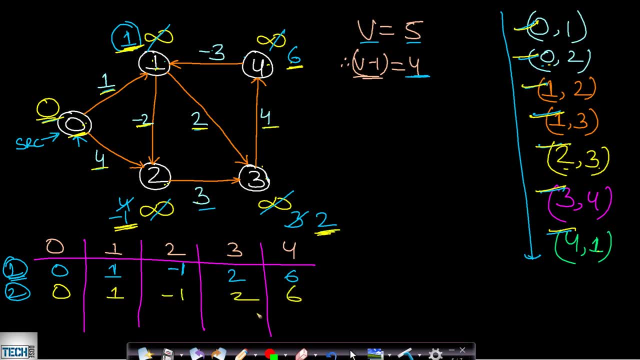 which has come is 0, 1 minus 1, 2 and 6.. now we had to relax actually four times in this case, but you can see that on the first time relaxation we had certain value. on the second time relaxation, we have certain value, and both the values are exactly the same. so whenever we find that these two 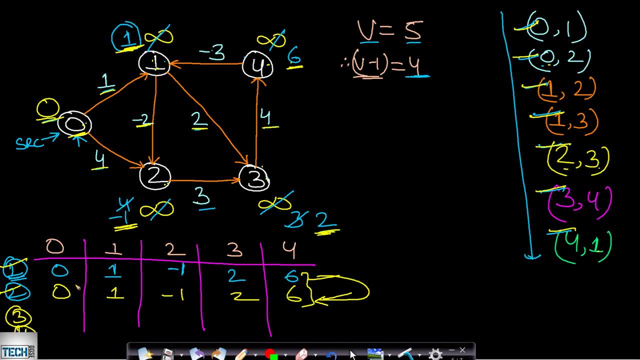 iterations, that is, two consecutive iterations, are the same values, that is, the same exact values for all the nodes. then we can say that it has been relaxed and we cannot relax it further. so in this case we can stop after relaxing for two times. okay, so this will give us the answer. so the shortest path from 0 to 3 will be equals to 2 and 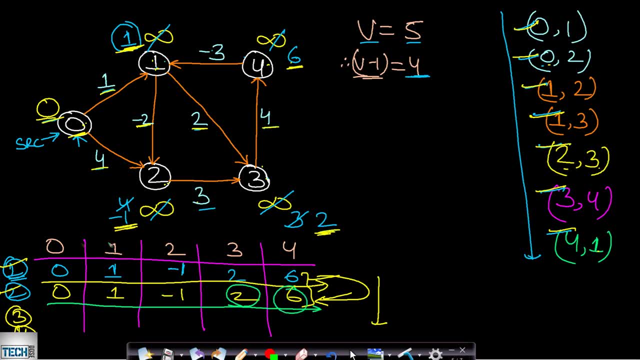 from 0 to 4 will be equals to 6, and similarly we can find from 0 to 1 and 0 to 2, so this will give us the answer. we don't need to relax for four times. so by seeing this, you can understand that. 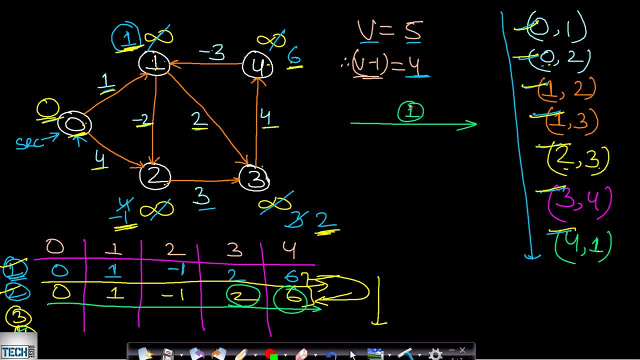 if certain step- relaxation- is having at least one node updated with a new shortest value, then definitely you will have to follow the next step- relaxation. otherwise, if a certain step is having no nodes updated, that is no shortest path you have found for a single scan, that is, for a 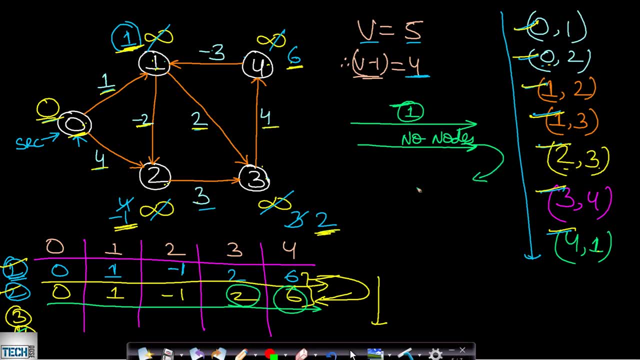 single step- relaxation- then in the next step as well, you will be performing the same relaxation types, that is, relaxing the same edges, and so you will definitely find no nodes to relax. therefore, it is wise that if, in a certain step, you are not finding any nodes which can be relaxed, 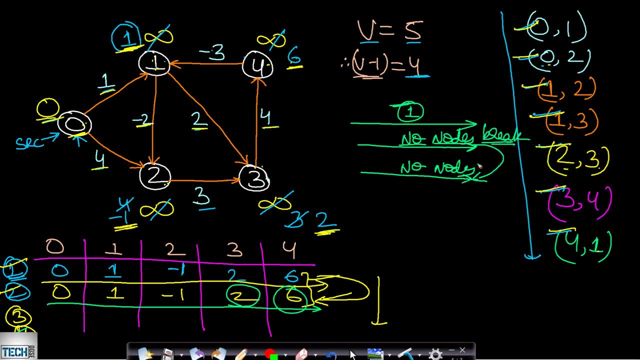 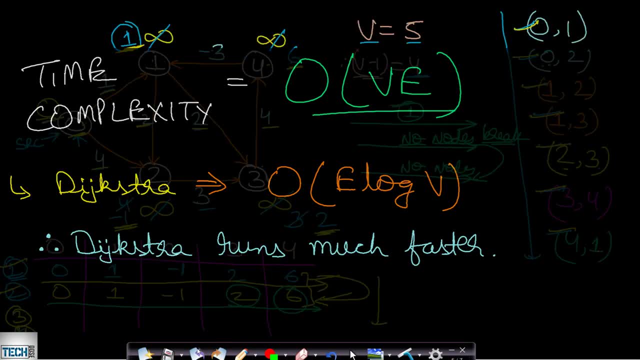 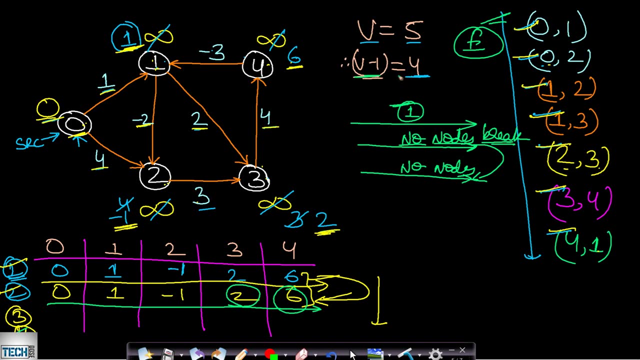 then you can break out here. so this will improve your time complexity as well. now, what will be the time complexity for this algorithm? it will be equals to order of ve. why? because we are relaxing e number of edges and we are relaxing all the edges for v minus 1 times. so 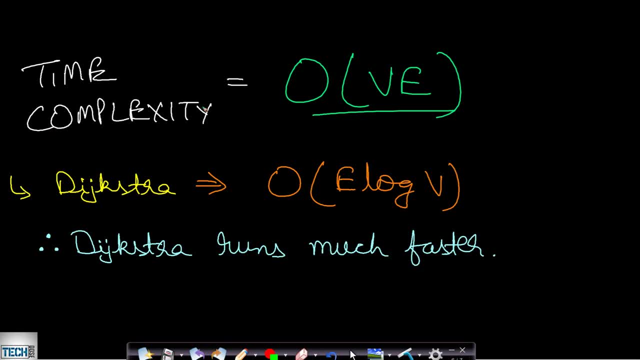 that is what we are doing now. we are relaxing all the edges for v minus 1 times. so that is time complexity will be order of ve. now you can see that this is far more than the dexter algorithm time complexity, which can go to e log v. so dexter runs much faster than the bellman ford algorithm. 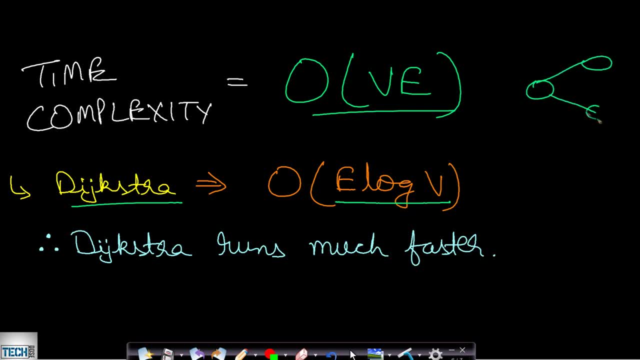 therefore, if you are sure that your graph will not be having any negative age, then you will definitely apply dexter algorithm, since it has much lower time complexity of e log v. otherwise, if you are not sure about it, then you can apply bellman ford. and if your graph is undirected graph. 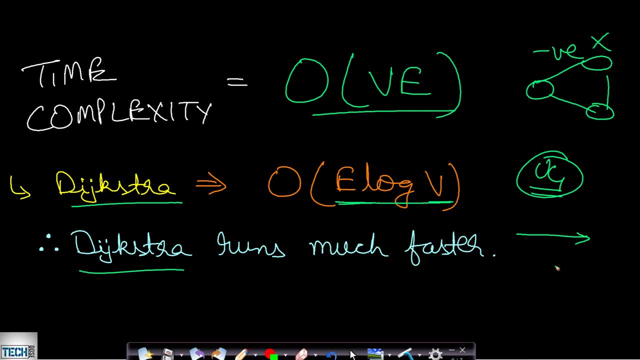 then definitely you can scan all the edges of the graph and see if any of the edge is having a negative edge weight. if it is true, then none of these algorithms will work. otherwise, if all the edges are positive, then definitely it will be having shortest path to all the vertices, and so 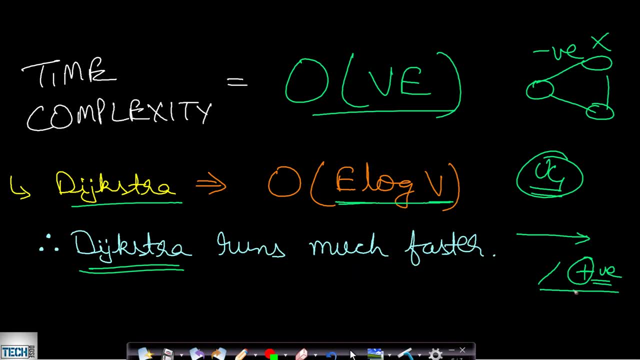 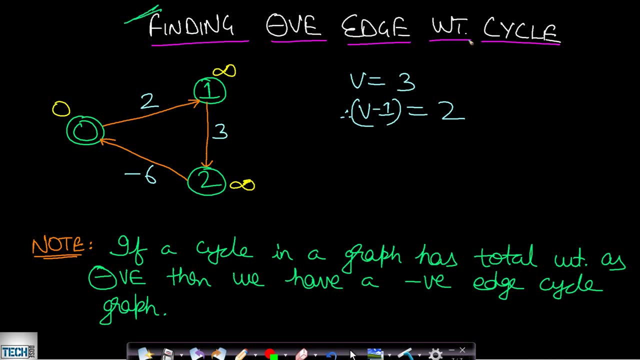 you can apply dexter algorithm and solve this problem faster. so this is one more optimization. now this was the last point which i had to say, finding negative edge weight cycle. so i had already explained what is a negative edge weight cycle. let us say, here we have three number of vertices. okay, so we will be relaxing it for two times. 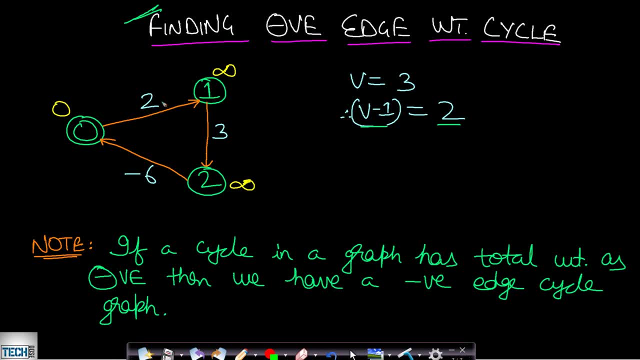 now from zero. what is the weight to this one? it is two. so the cost from zero to one will be equals to two, because zero is the source node, and from source to one it will be having the minimum cost as 0, 2.. now we will relax the next edge, which is from 1 to 2. it will be 2 plus 3, which will be 5.. now from 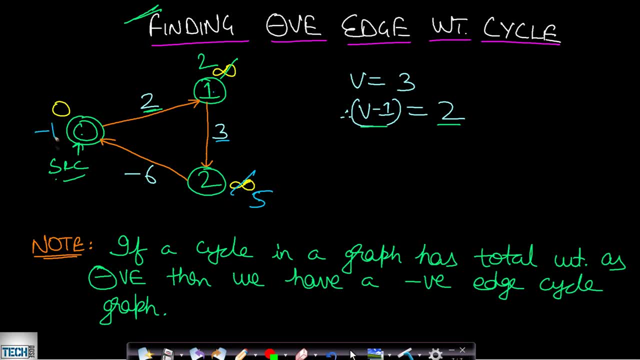 2 to 0, it will be 5 plus minus 6, which will be minus 1. so we have done one iteration. okay. now we will perform the second iteration. in this case, from 0 to 1, the cost will be minus 1 plus this 2. 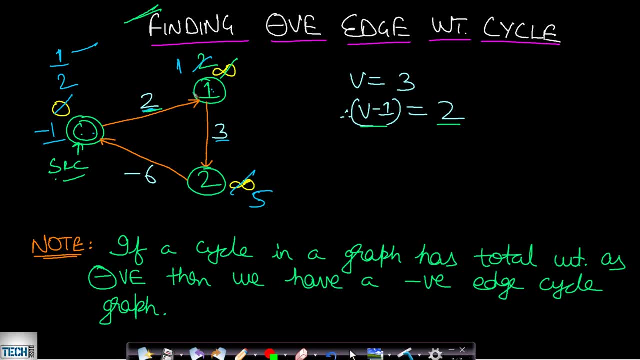 which will be 1.. now, from 1 to 2, the cost will be 1 plus 3, which will be 4. from 2 to 0, the cost will be 4 plus minus 6, which will be minus 2.. now we have relaxed 2 times, which is v minus 1 times, and 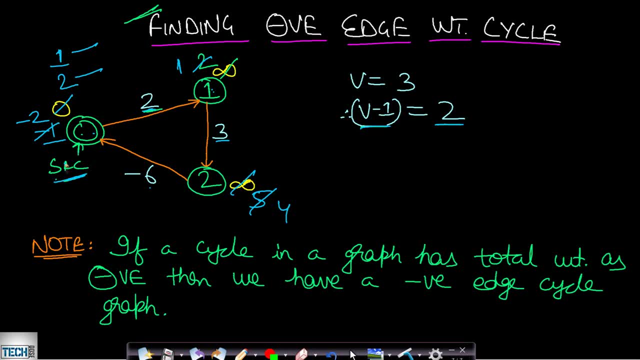 so we should have found all the shortest path starting from this source node. okay, so now we will try to relax one more time. so we will relax the third time. in the third time we should not find any new shortest path now. we will start from this: 0. the cost is minus 2. 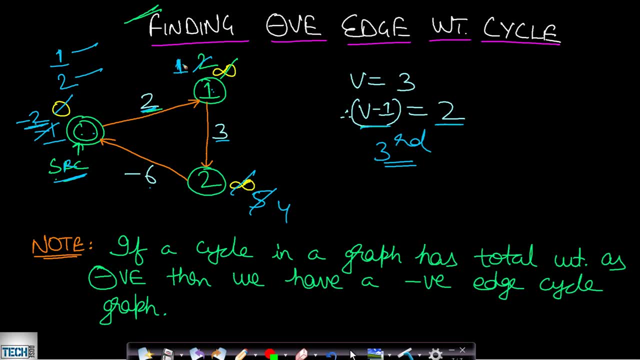 minus 2 plus 2 is 0, and here the cost is 1.. so now your new cost is 0.. you can see that you have found a new, shortest cost in order to reach from 0 to 1. okay, so this should not have been the case. actually, you should have found all the shortest cost in v minus 1 times. 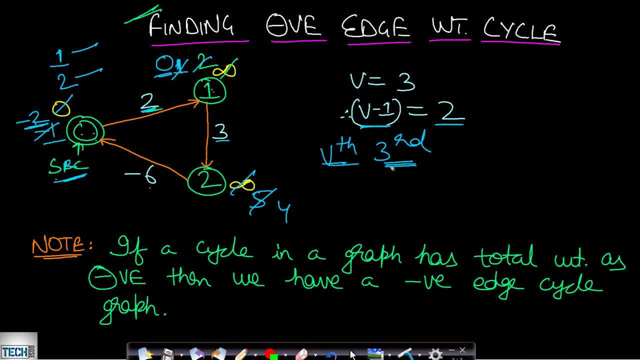 but in the vth time- that is, the third time- you are finding a new, shortest path, and so this will confirm that your graph is having negative edge weight cycle. so if a cycle in a graph has total weight as negative, then we have a negative edge weight. 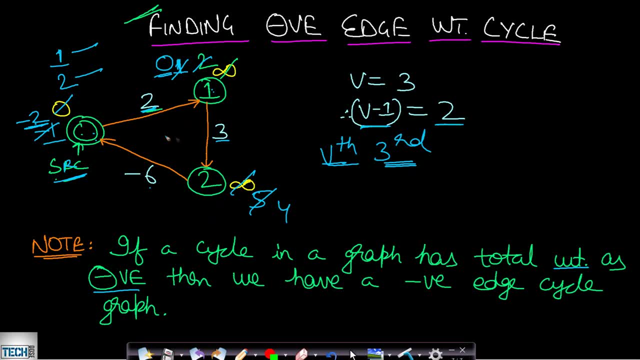 edge cycle graph. so this i have already explained. like in this case the edge weight was 2 plus 3 plus minus 6, so the total cost will be 2 plus 3 plus minus 6, which will be equals to minus 1. so if you make one cycle, then your total cost will be decreased by 1 if you make the second cycle. 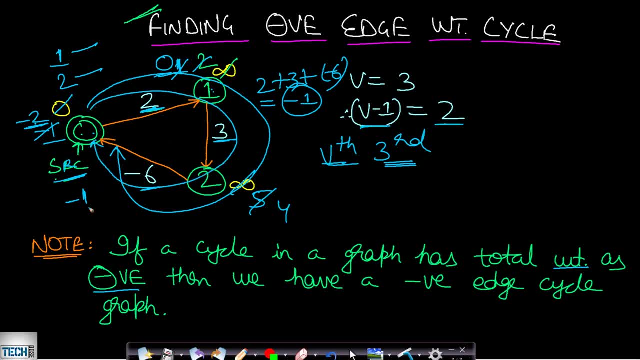 from this 0 to 0, then your cost will decrease by again minus 1 and it will now become minus 2. so this is what is happening here. okay, so that is why when you have a negative edge weight cycle, then you will never be able to find the shortest path using Dijkstra or Bellman-Ford algorithm. 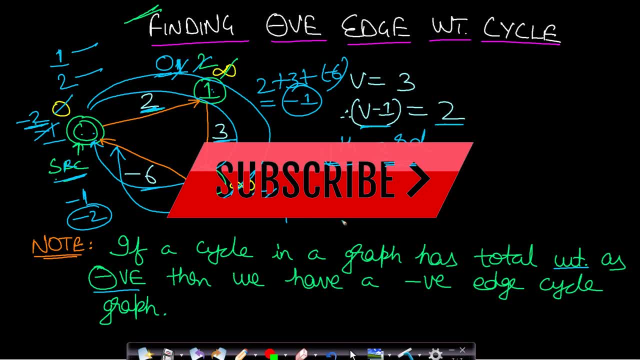 so i hope you got the understanding now. in the next video, i will be showing you the code implementation, along with the dry run of some good example. okay, if you have any doubt, then feel free to comment below and i'll try to help you as soon as possible. like and share our video and subscribe.